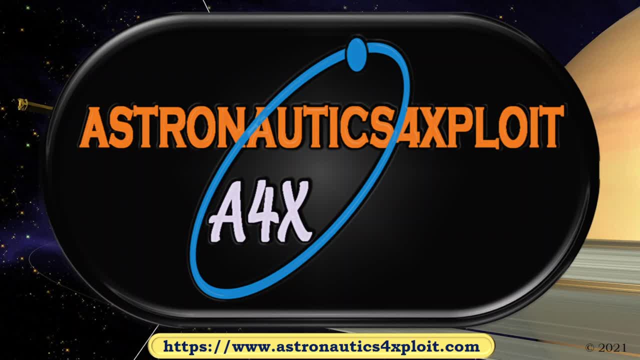 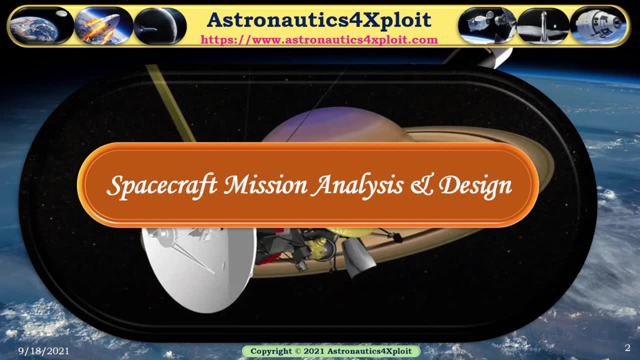 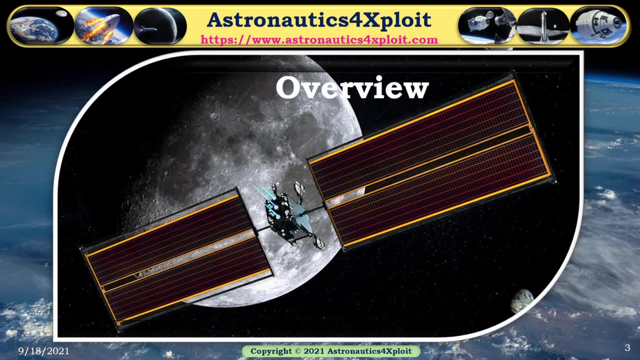 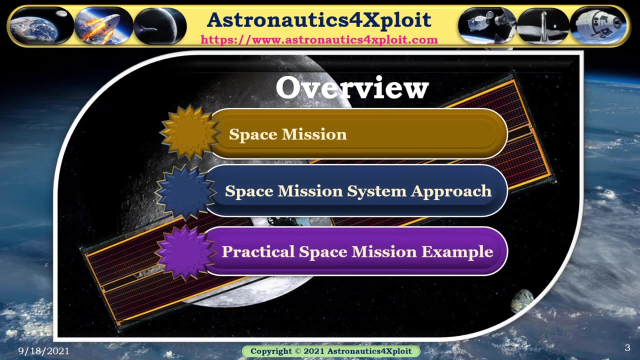 Hello, welcome to Astronautics for Exploit. Hi, I'm Dr Ayinshola Ogundile and I will be presenting spacecraft mission analysis and design. The overview of my presentation is as follows: Space mission, space mission system approach and practical space mission example. 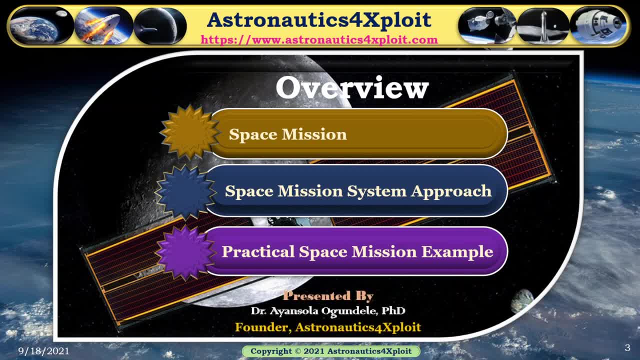 The new space race is opening the doors to a world of many possibilities and is a driver for increasing public interest in space exploration and, recently, space tourism. It has brought in a fast-moving Silicon Valley and product-led paradigm to a sector that was previously the government's domain. Space exploration is offering a 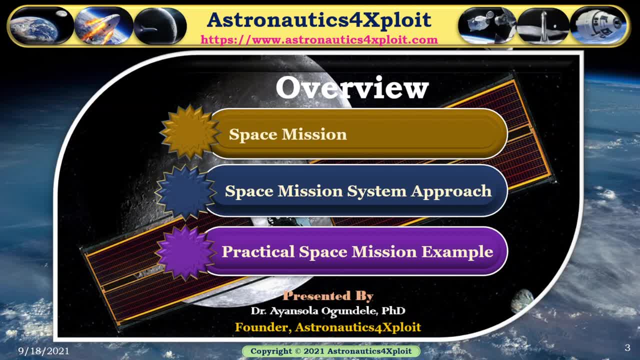 lot of benefits to the humankind and advancing our knowledge about the universe and its composition. Examples of what have been achieved through space exploration are launching of Sputnik 1, Yuri Gagarin's first flight in space, the Apollo missions to the moon. 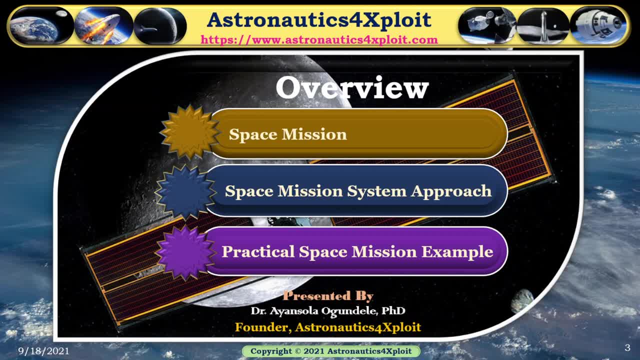 the shuttle program, the Hubble Space Telescope launch, maintenance on a Hobbit and, finally, the assembly exploitation of the International Space Station. These challenges were undertaken and are still being undertaken by the government and private investors. Increasing interest on space exploration is necessitating the need to have a well-planned and executed space mission analysis and design. 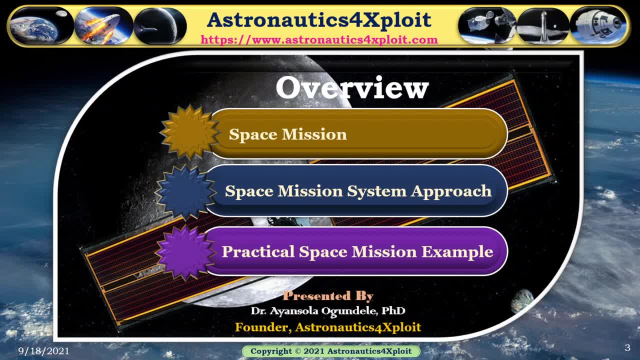 Generally, the mission design process begins with a statement of the mission, objectives, mission classification and programmatic constraints. Conceptualizing and executing space missions calls for creative thinking coupled with careful and conservative implementation. The engineers and scientists who design such missions must master 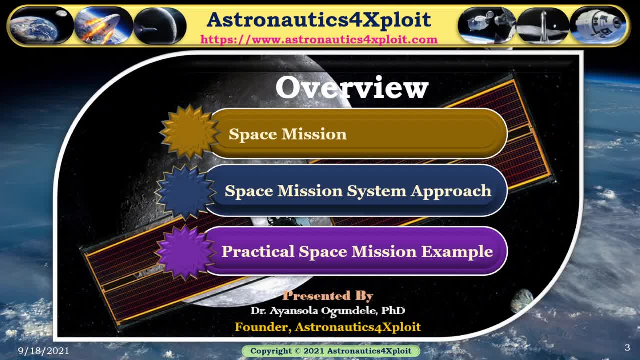 a wide dynamic range of techniques, from brainstorming to design reviews. Operating in space has never been easy and the better: faster, cheaper. mandate imposed by today's over-constrained budget has created new complications. Starting with the whole important mission objective, top functional requirements are: 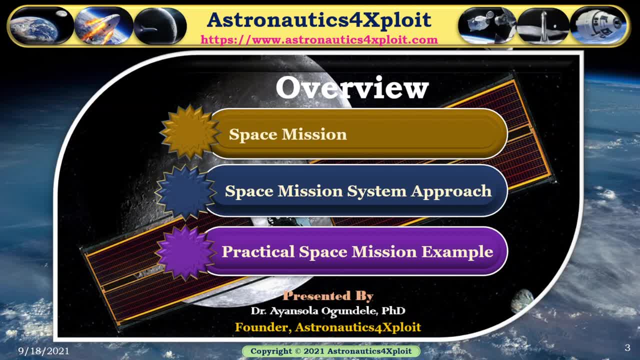 established, Taking into consideration the available capabilities and the imposed constraints. a solution, that is, the mission design, is synthesized by an iterative process of analysis and design. Subordinary requirements on the launch vehicle spacecraft and the subsystems, along with mission operations, are then flowed down from the top level. 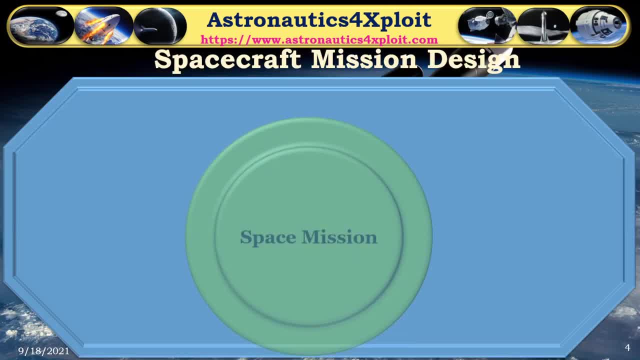 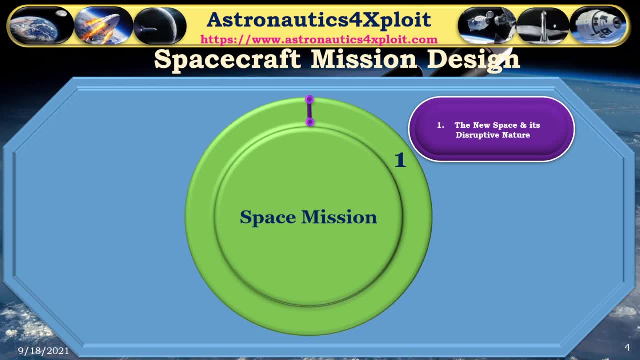 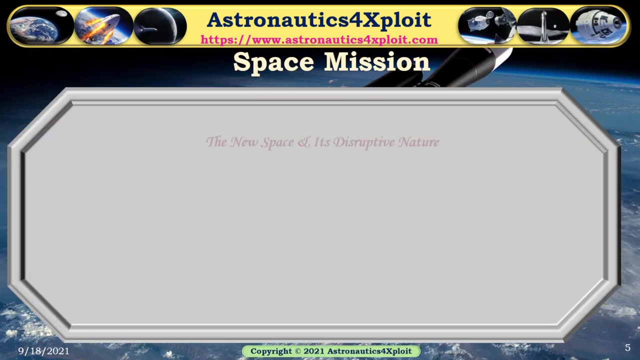 requirements Space Mission. Space mission is divided into the following: the new space and its destructive nature. space mission life cycle element of a space mission and role of this of spacecraft mission design engineer in an evolving world. the new space and its destructive nature. the advent of new space companies, such as spacex. 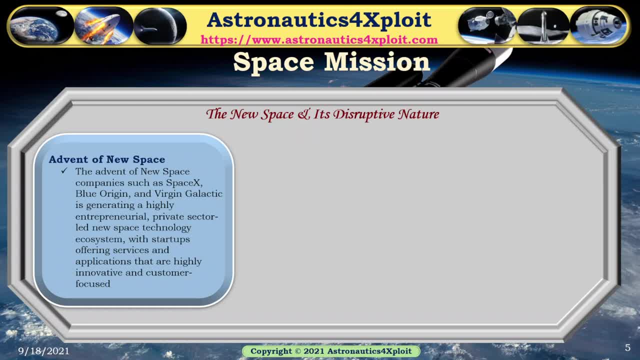 space and its destructive nature. the advent of new space companies such as spacex, blue origin and fadging galactic is generating a highly entrepreneurial, private sector-led new space technology ecosystem, with startups offering services and applications that are highly innovative and customer focused. Morgan Stanley, which predicts that the global space industry will generate revenue upwards of 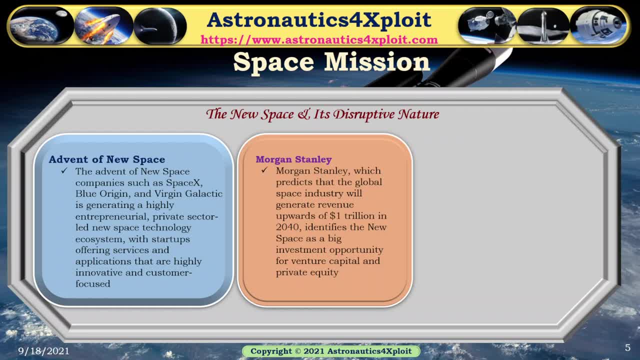 1 trillion dollars in 2040, identifying the potential for the future of space. and the future of space identifies the new space as a big investment opportunity for venture capital and private equity. the new space ecosystem and its constellation of space tech startups and unicorns ready to. 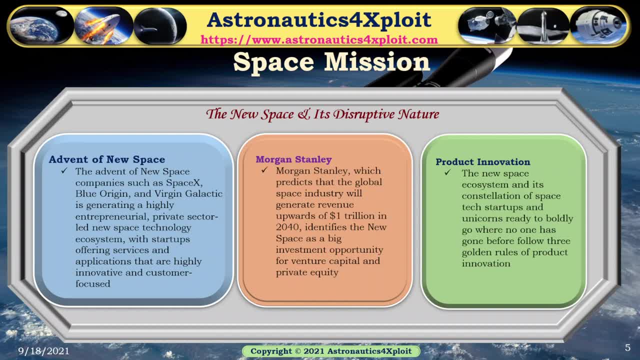 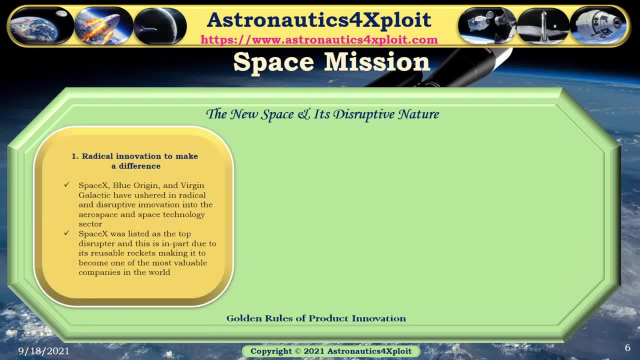 boldly go where no one has gone before. follow three golden rules of product innovation. the new one is radical innovation. to make a difference, spacex, blue origin and fadging galactic have ushered in radical and destructive innovation into the aerospace and space technology sector. spacex was listed as the top disruptor and this is in part due to its reusable rockets. 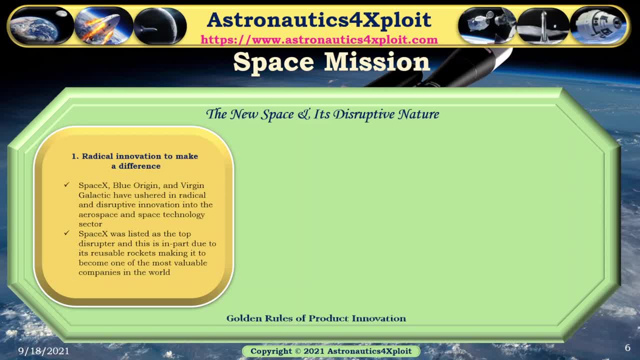 making it to become one of the most valuable companies in the world. The second one is lower barriers to mass satellite production, launch and space tourism. Fadging galactic and blue origin are stated that they want to lower barriers to mass adoption of space travel. 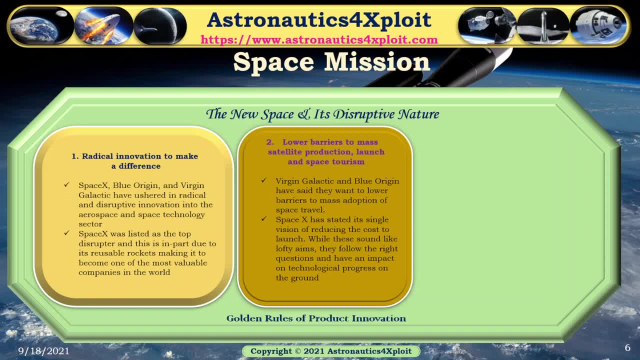 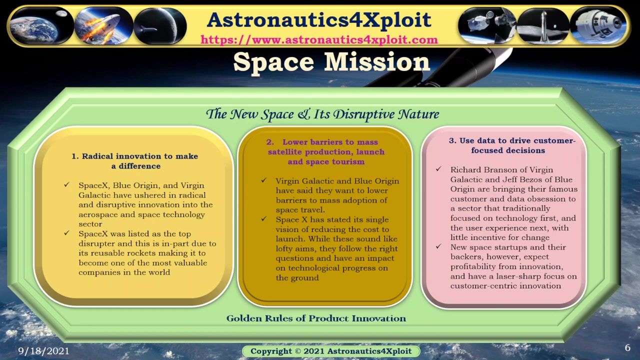 facilitating continuous space tourism. Spacex has stated a single vision of reducing the cost of launch. while they sound like lofty imps, they follow the rest of the brain, the right questions and have an impact on technological progress on the ground. The third one is use data to drive customer-focused decisions which are bracing of Farging Galactic. 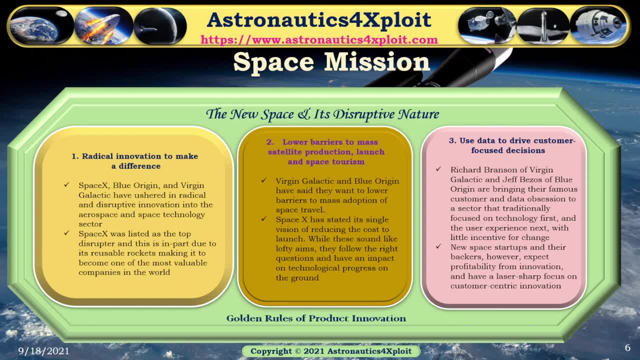 and Jeff Bezos of Blue Origin are bringing their famous customer and data obsession to a sector that traditionally focused on technology first and the usual experience next, with little incentive for change. New space startups and their backers, however, expect profitability from innovation and have 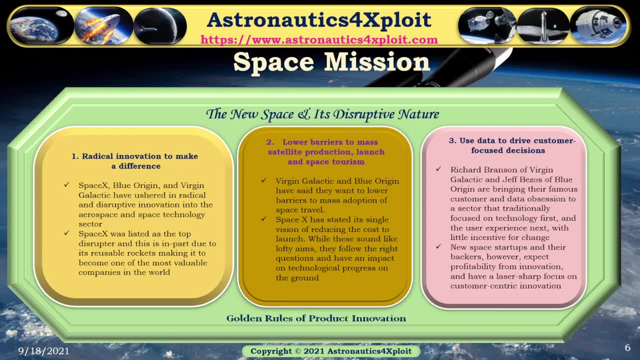 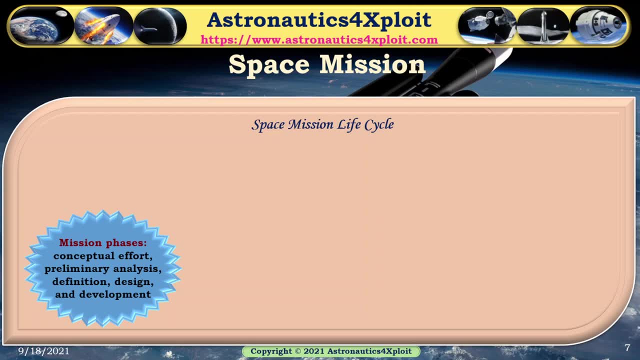 a laser-sharp focus on customer-centric innovation. Space Mission Life Cycle Mission phases are divided as follows: Conceptual Effort, Preliminary Analysis, Definition, Design and Development. It starts from Preface A, which is the conceptual study phase, And the conceptual study phase is the phase that is prior to Phase A. 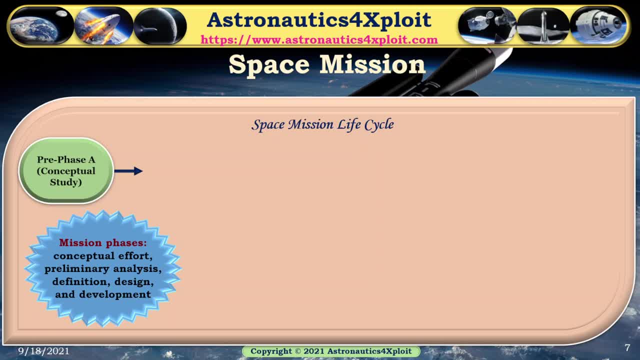 The conceptual research relates to abstract concepts and ideas. It doesn't involve practical experimentation, But instead relies on the researcher analysing available information on a given topic. Conceptual research is a methodology where hand research is conducted by observing and analysing already present information on a given topic. 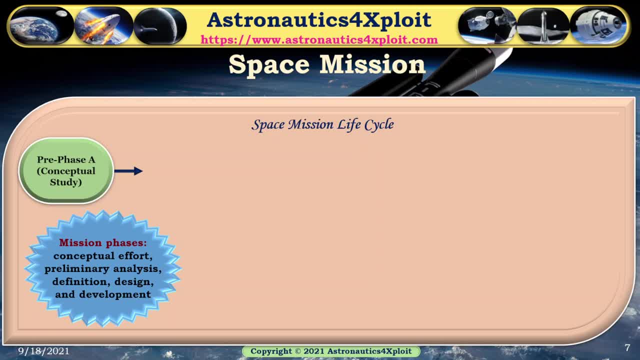 It actually focuses on the concept of theory that explains or describes the phenomena, as well as the concept of the project. Another aspect is Phase A, which is the Preliminary Analysis. So after the conceptual study, we have the Preliminary Analysis. 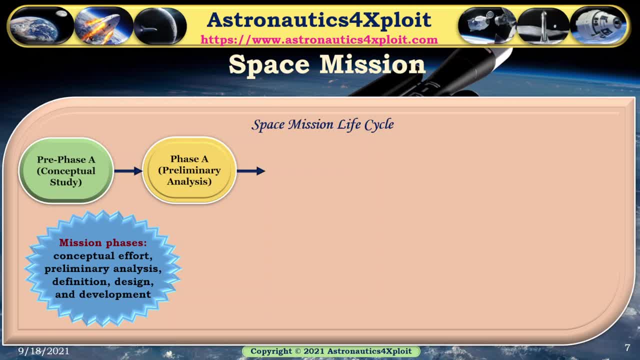 The project creates a preliminary design and project plan as a proof of concept, specifying what to build, when to launch, the course the spacecraft will take and what is to be during the cruise, when the spacecraft will reach the target and what operations will. 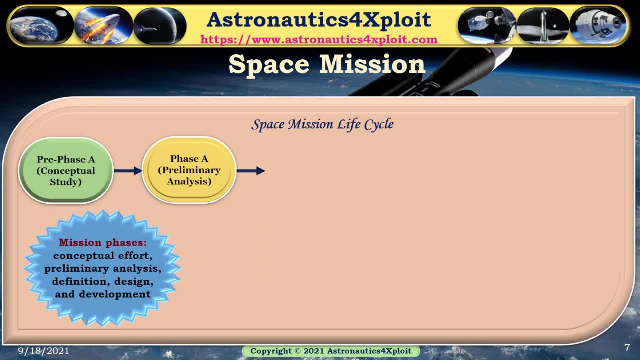 be carried out. So the preliminary plan also addresses build-forces-buy decisions: What spacecraft instruments are needed, where system tests will be performed, who performs the mission operations, what ground data system capabilities are required and who the experimenters are. So after this we have the phase B definition. 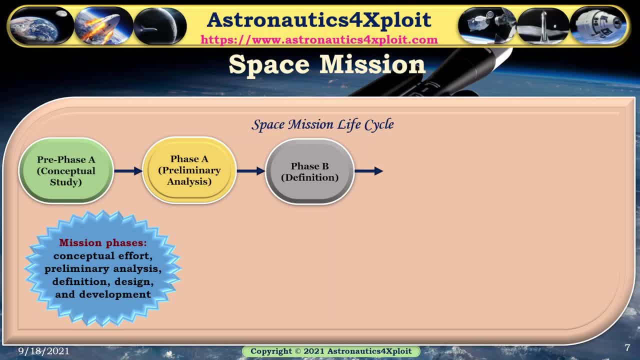 The definition phase converts the preliminary plan into a baseline technical solution. Requirements are defined, schedules are determined and specifications are prepared so as to initiate system design and development. Major reviews commonly conducted as part of the definition phase are system requirements, the system design review and non-advocate review. 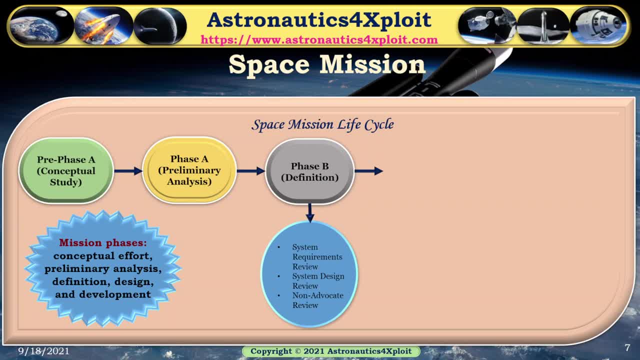 The proposed experiments are divided into two classes, based on facilities and experimenters. The facilities form teams around the designated set of hardware, and facilities are selected based on existing resources and past performance. Then experimenters were specified in the preliminary plan. However, in the field they are encouraged to respond with modifications and to step 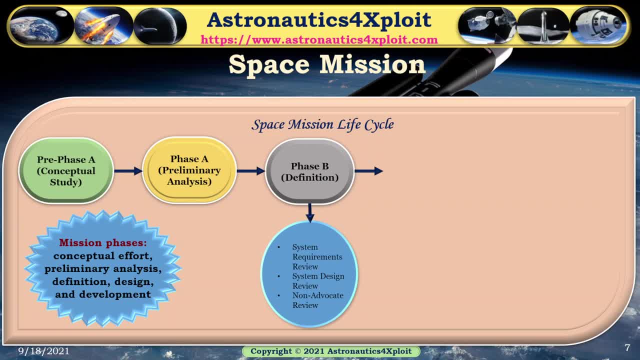 forward with their own ideas. The ideas could include the addition of another experiment. So after phase B, we have the phase C and D, which is the design and development- During the design and development phase, schedules are negotiated- and the space flight system. 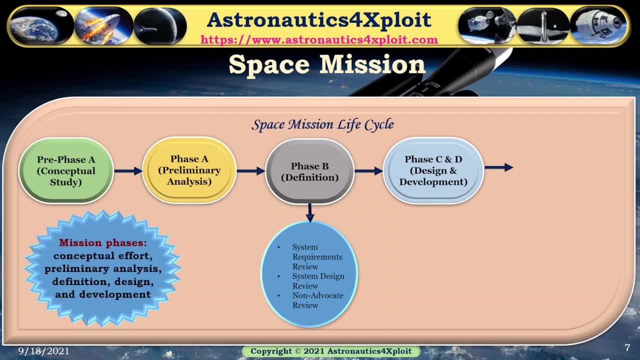 is designed and developed. The phase begins with building and development. The design and development phase is the phase of design and development. After the phase C and D, we have the operations phase, which is the mission operation and data analysis. Operation phase is also called mission operation and data analysis. 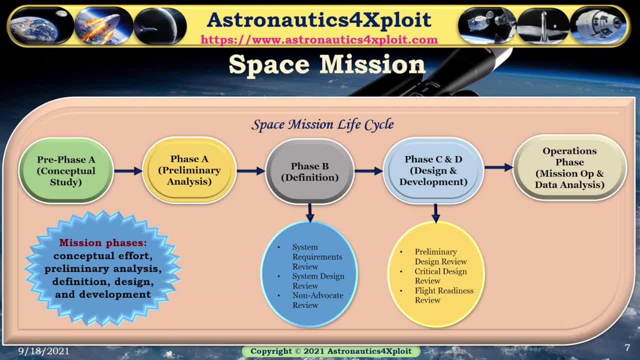 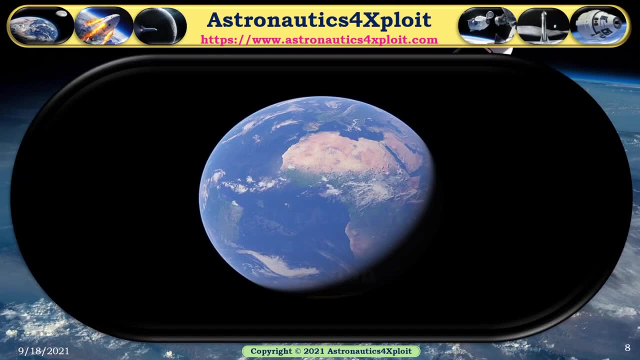 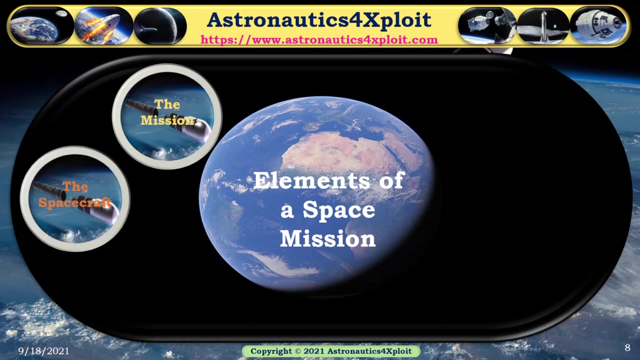 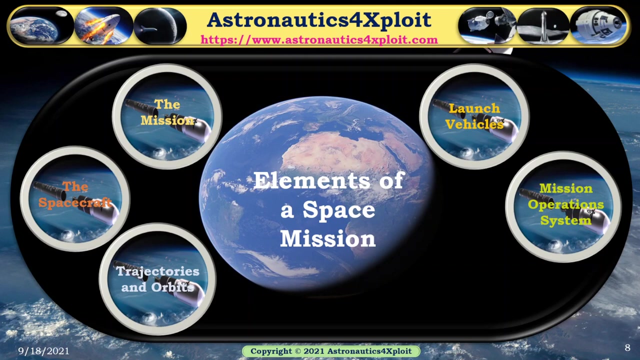 It includes flying the spacecraft and obtaining science data for which the mission will be designed. We have the preliminary mission and the extended mission as subsets of the operations phase. Elements of a space mission: The mission, spacecraft trajectories and orbits, launch vehicles, mission operations system. 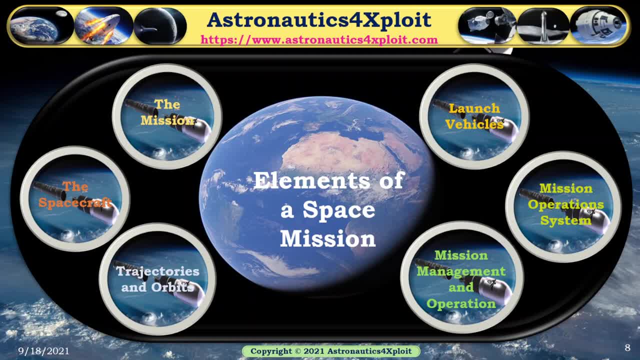 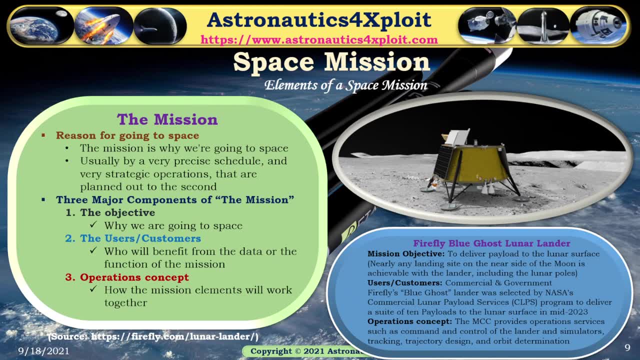 mission, management and operations. These are the six elements of a space mission: The Mission: The mission is why we are going to space, usually by a very precise schedule and very strategic operations that are planned out. to the second, There are three major components of the mission, which are: the objective, which states the. 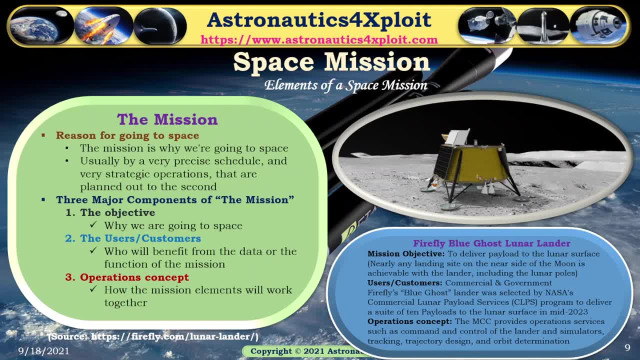 reason why we are going to space, The users or customers. customers who will benefit from the data or the function of the mission, and the operations concept, how the mission elements will work together. a typical example of the mission is given here. well, for the firefly blue ghost lorinander, the mission objective is to deliver payload to the 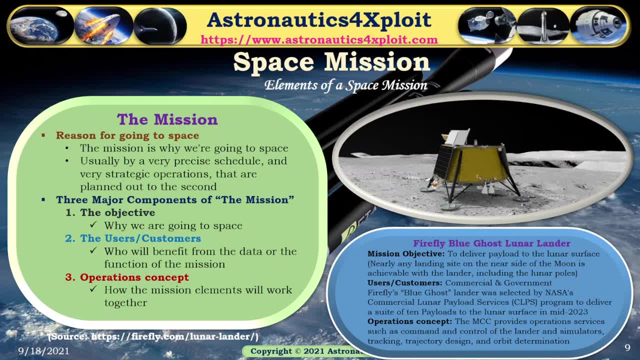 lunar surface. nearly any landing site on the near side of the moon is achievable with the lander, including the lunar poles. then we have the users and customers, commercial and government. the fireflies blue ghost ladder was selected by nasa's commercial lunar payload program in order to deliver a suite of 10 payloads to the lunar surface in the mid-2023. 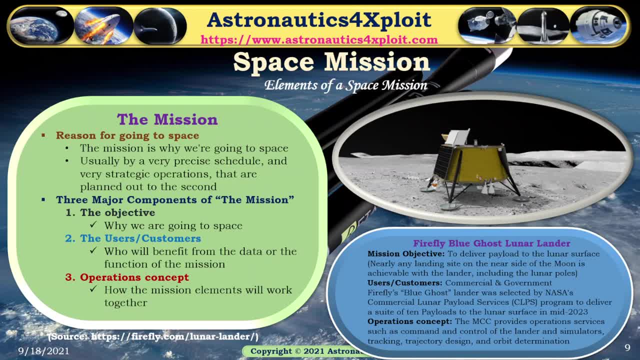 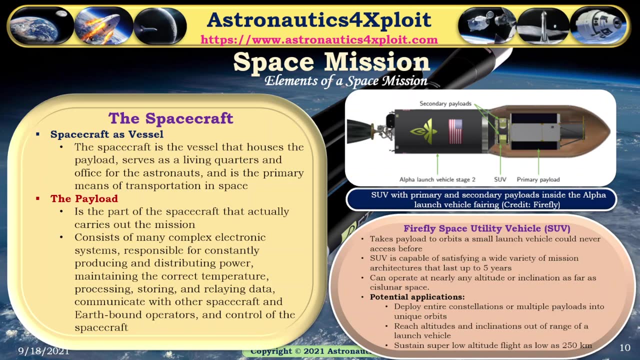 then we have the operations concept. the monitoring and control center provides operational services, such as command and control of the lander and simulators, tracking, trajectory design and orbit determination. the spacecraft: spacecraft is a vessel that houses the payload, serves as a living quarters and office for the astronauts, and is the primary means of transportation in space. 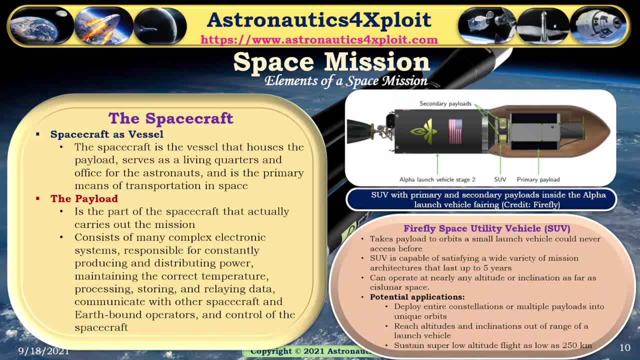 the payload is the part of the spacecraft that actually carries out the mission. it consists of many complex electronic systems responsible for constantly producing and distributing power, maintaining the core correct temperature, processing, storing and relaying data, communicating with other spacecraft and altri operators and control the spacecraft. this picture shows suv with primary and secondary. 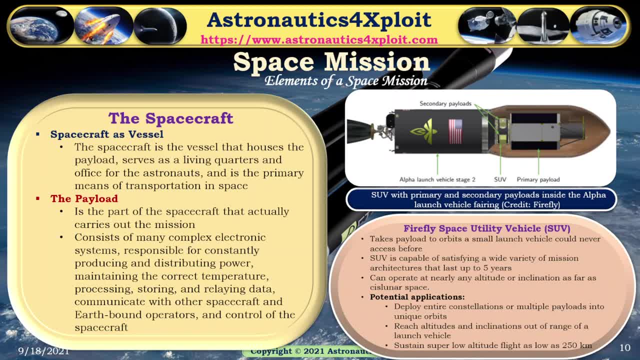 payloads inside the alpha lounger vehicle fair. so the it takes payload suv, takes pillar to orbits. actually it is capable matchyto the white variety of mission architectures which can last up to five years. The potential applications are to deploy entire constellations or multiple payloads into unique orbits, reach altitudes. 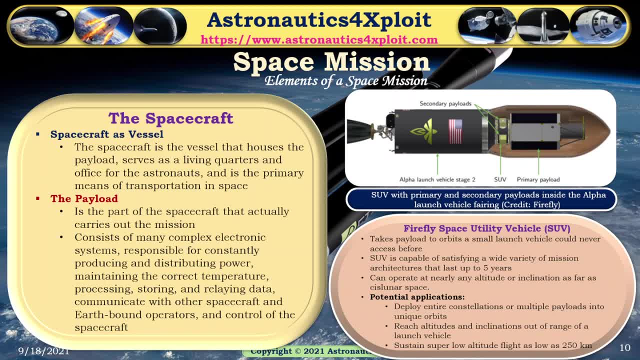 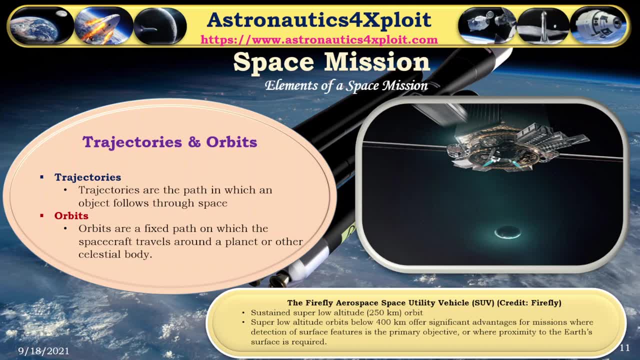 and inclinations out of range and sustain super-low altitude flight. Trajectory and Orbit Trajectory are the path in which an object follows through space. Orbits are a fixed path on which the spacecraft travels around a planet or other celestial body. This picture shows the Fairfly Aerospace Space Vehicle. 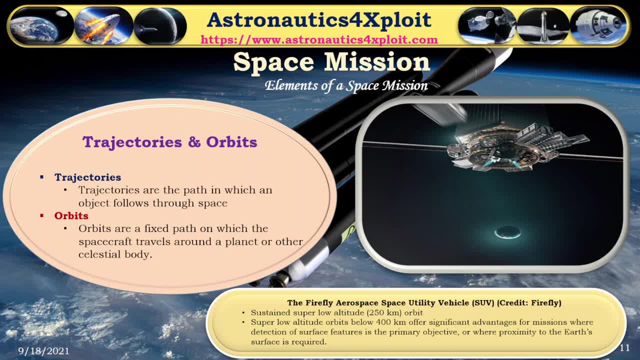 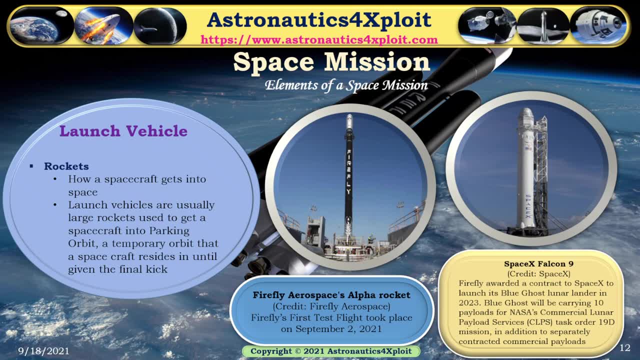 It sustains super-low altitude of 250 km orbit Launch Vehicle Rockets. How a spacecraft gets into space is being enabled through rockets. Launch vehicles are usually large rockets used to get a spacecraft into a parking orbit, A temporary orbit that a spacecraft resides in until given a final kick. 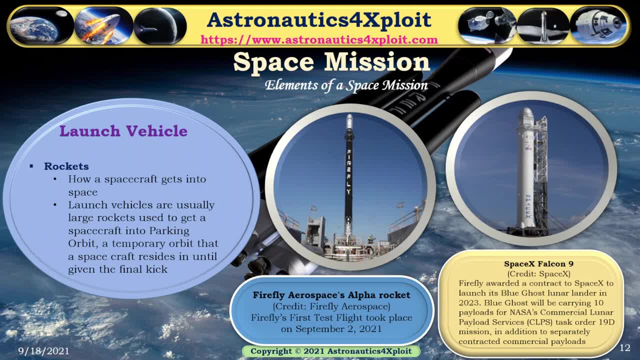 This picture shows two scenarios where a customer might request a well-established space launch organization to launch a spacecraft for him. like in the case of SpaceX, which launches satellites for people and also launches a spacecraft for the spacecraft itself, a company can launch its own satellite, which. 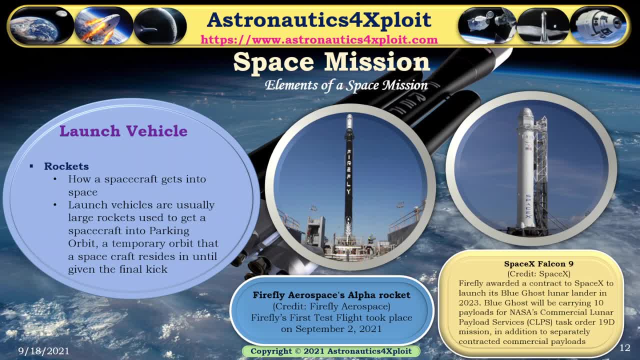 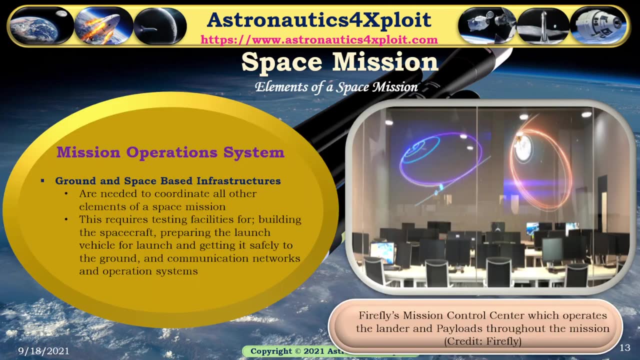 is shown in the pictures here, where we have the Fairfly Aerospace Alpha rocket and we have the SpaceX Falcon 9.. Fairfly awarded a contract to SpaceX in order to launch its Blue Ghost Lowlander in 2023.. Mission Operation System: Ground and Space-Based. 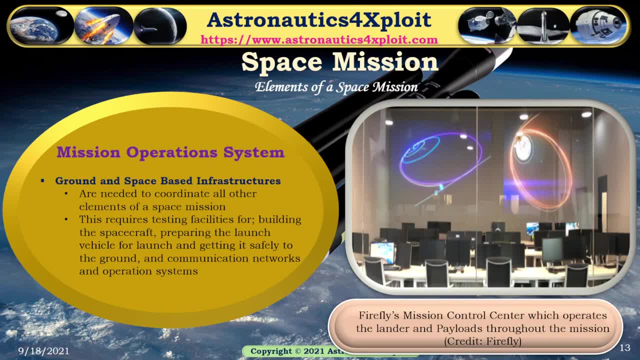 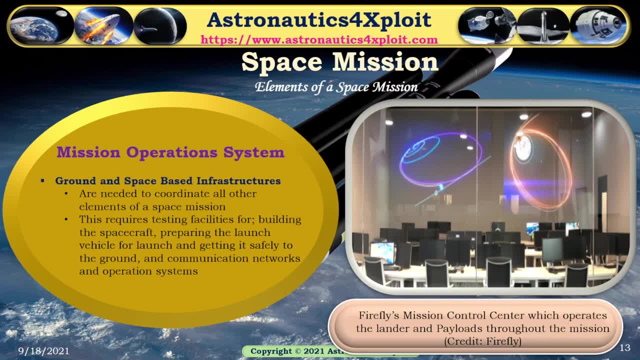 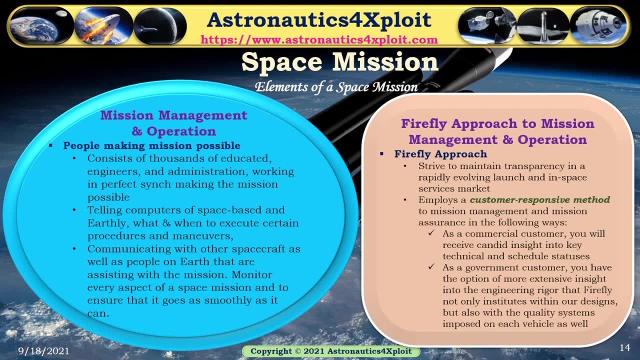 spacecraft, preparing the launch vehicle for launch and getting it safely to the ground, and communication networks and operation systems. Mission Management and Operation. It consists of thousands of educated engineers and administration working in perfect sync, making the mission possible, telling the computers of space based and earthly what and when to execute certain procedures and maneuvers. 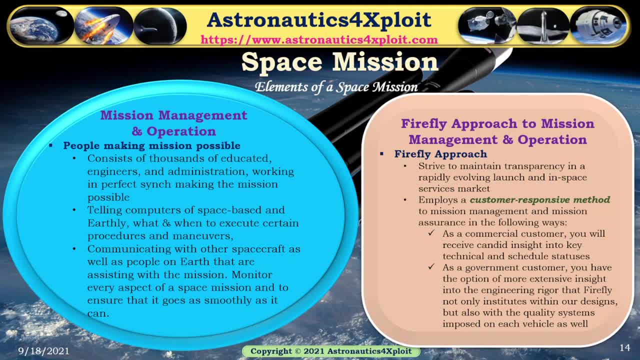 communicating with other spacecraft, as well as people on earth that are assisting with the mission. monitor every aspect of a space mission and to ensure that it goes as smoothly as it can. The approach to mission management and operation of Fairfly is stated here. strive to maintain transparency in the rapidly evolving launch and in-space services. 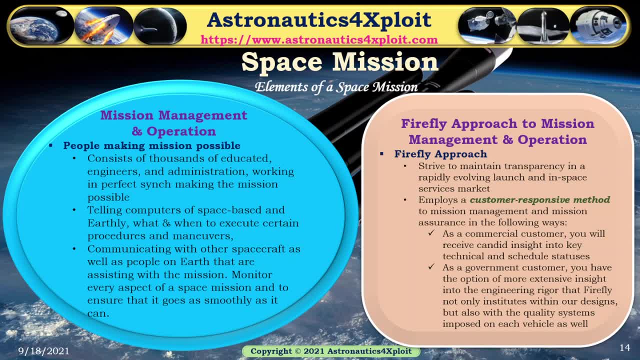 and to ensure that the mission is successful. The mission management and operation of the mission management and operation of the mission management and operation of the mission management and mission assurance in the following ways: As a commercial customer- one will have the ability to have an insight into key technical and schedule statuses- and as a government customer. 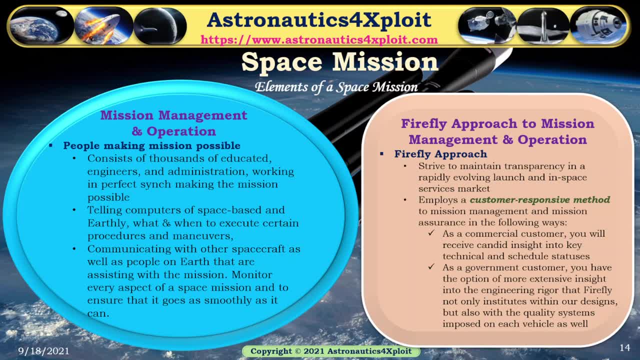 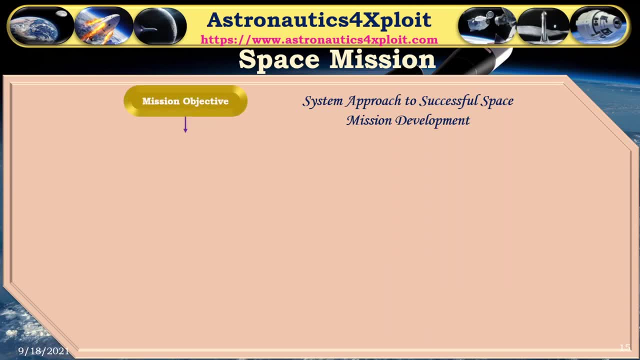 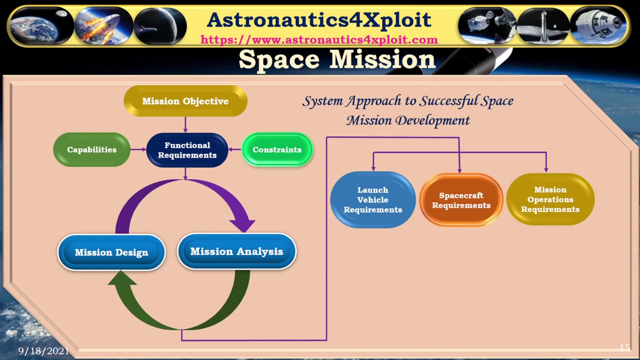 one will have the option of more extensive insight System Approach to Successful Space Mission Development. We have the mission objectives, which goes into the functional requirements. Then the capabilities and constraints comes into the functional requirements. The output of functional requirements goes to mission design and mission analysis. The output of mission design and mission analysis. 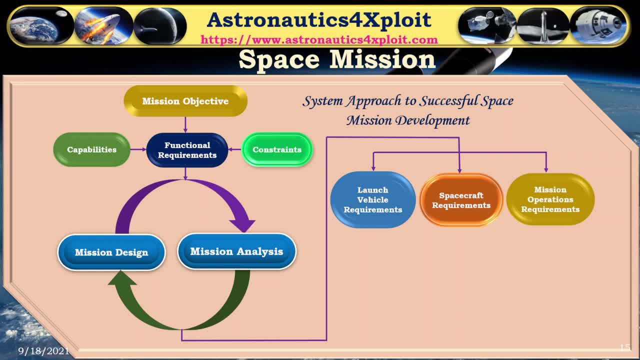 goes to launch vehicle requirements, spacecraft requirements and mission operations requirements. Then spacecraft requirements goes into block power flow and signal flow diagrams, the specs interface control documents, ability configurations and launch configuration. This shows the requirements flow down from the mission objectives. 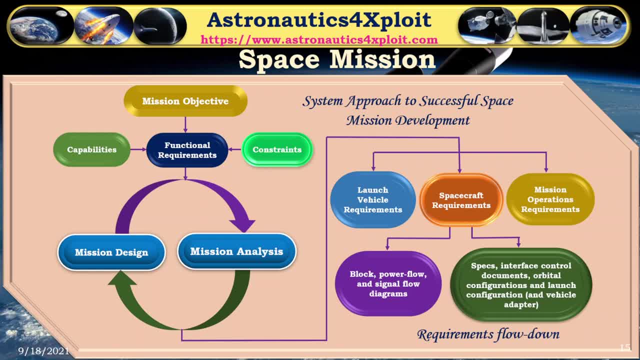 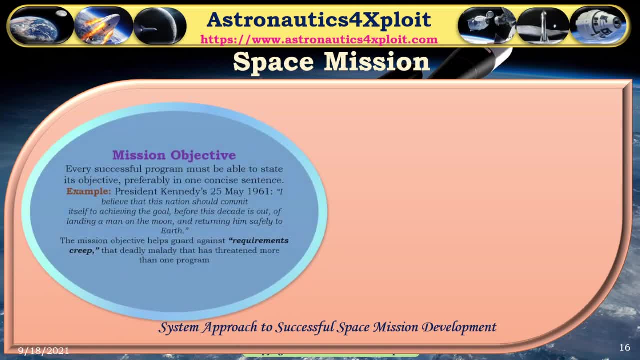 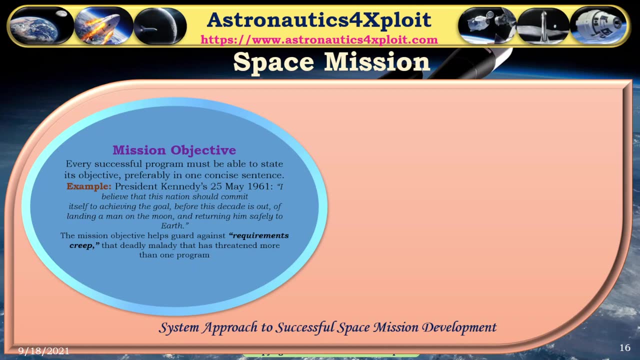 into the block power flow and signal flow diagram and configurations. 瞯ы infringement Notifications, management and operations of Phase Design and Gladi 그�賽 Mission Objective: Every successful program must be able to state its objective, preferably in one concise sentence. 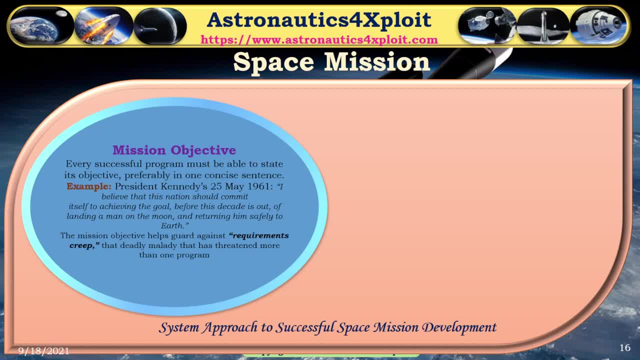 For example, President Kennedy on 25 May 1961 said: I believe that this nation should commit itself to achieving the goal, before this decade is out, of landing a man on the moon and returning him safely to Earth. The mission objective helps guide against requirements creep. 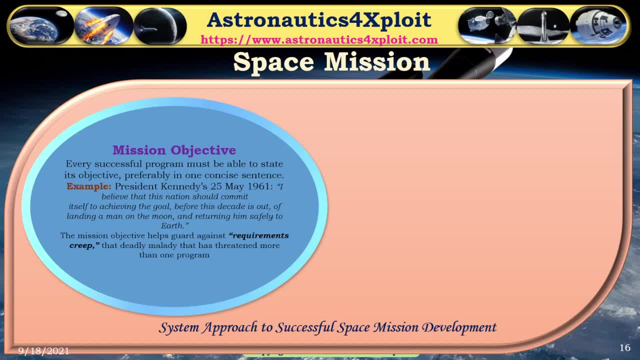 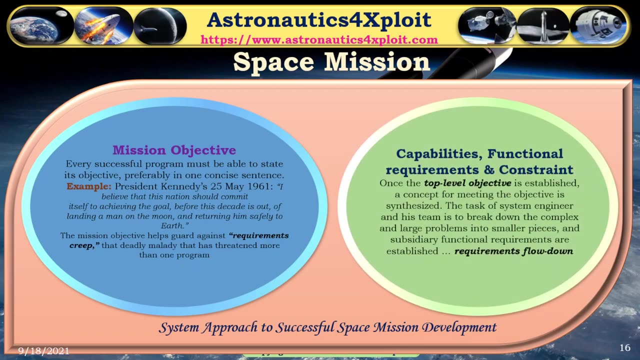 the deadly malady that has threatened more than one program. So through the mission statement, the aim was achieved, as stated by President Kennedy. Capabilities, Functional Requirements and Constraints: Once the top-level objective is established, a concept for meeting the objective is synthesized. 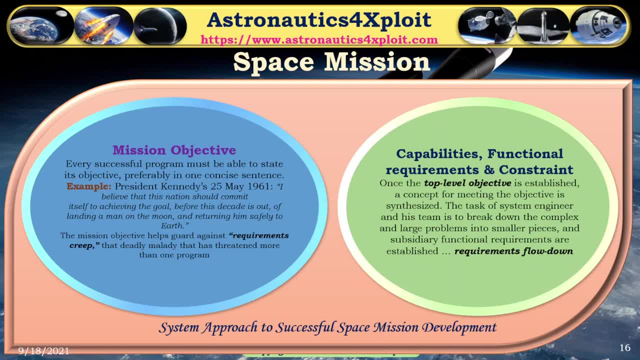 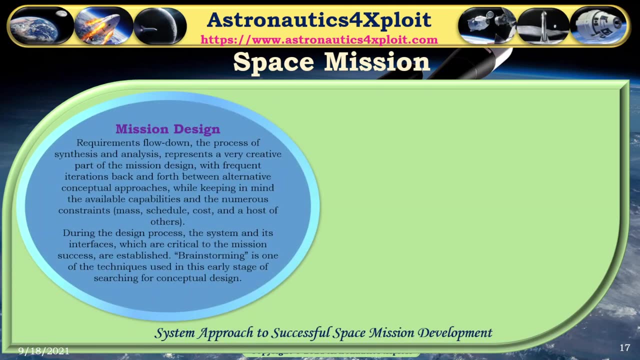 The task of system engineer and his team is to break down the complex and large problems into smaller pieces, and subsidiary functional requirements are established. This refers to Requirements Flowdown- Mission Design, Requirements Flowdown- the process of synthesis and analysis- represents a very creative part of the mission design. 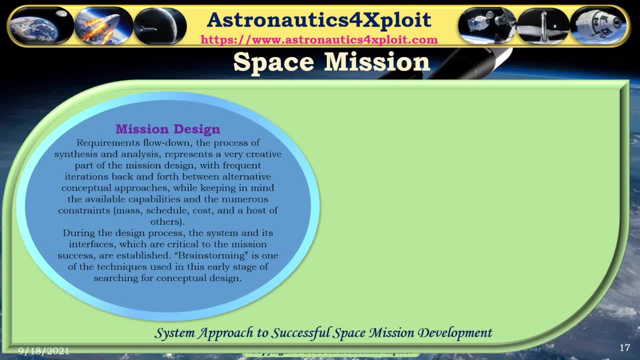 We frequent iterations back and forth between alternative conceptual approaches. while keeping in mind the available capabilities and the numerous constraints, such as the mass schedule, cost and a host of hurdles During the design process, the system and its interfaces, which are critical to the mission's success, are established. 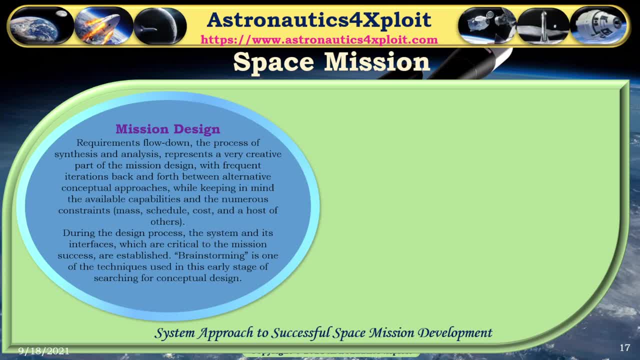 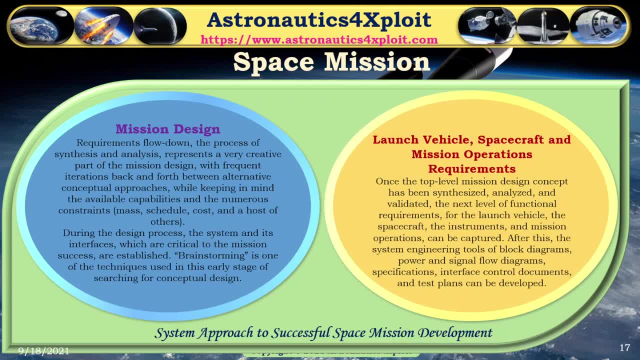 Brainstorming is one of the techniques used in this early stage of searching for conceptual design, Launch Vehicle, Spacecraft and Mission Operations. Once the top-level mission design concept has been synthesized, analysed and validated, the next level of functional requirements for the launch vehicle, the spacecraft. 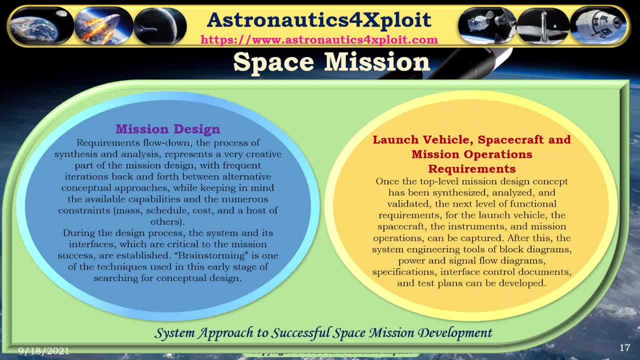 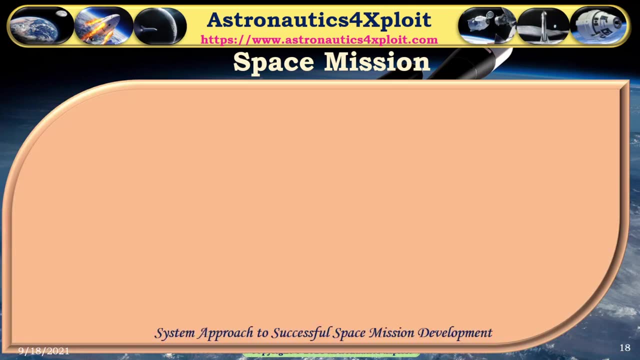 the instrument and mission operations can be captured. After this, the System Engineering source bloc, flame diagrams, power and signal flow diagrams, specifications, interface control documents, the launch vehicle, the spacecraft and mission operations can be captured and test plans can be developed. the program management: a key to successful program management. 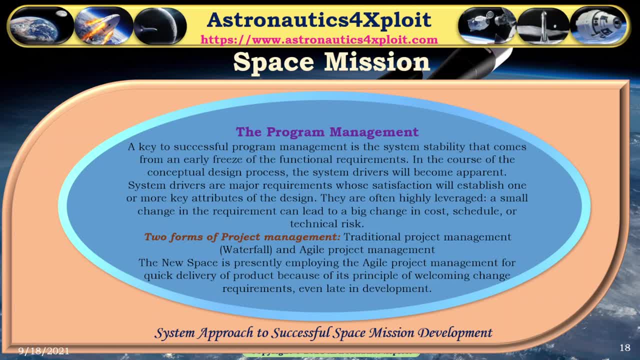 is the system stability that comes from an early phrase of the functional requirements. in the course of the conceptual design process the system drivers will become operant system drivers. there are major requirements whose satisfaction will establish one or more key attributes of the design. they are often highly leveraged. a small change in requirement can lead 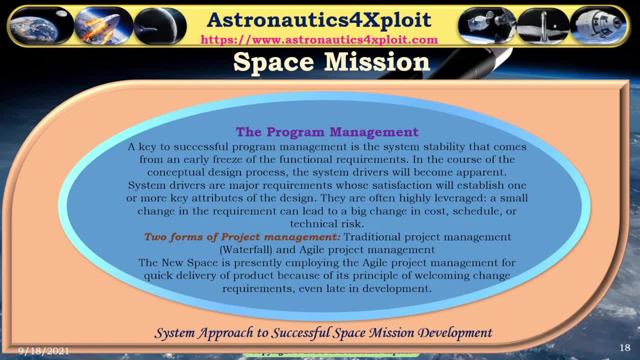 to a big change in cost schedule or technical risk. there are two forms of project management: traditional project management, which is reversed as waterfall, and the agile project management. the new space is presently employing the agile project management for quick delivery of product because of its principle of welcoming change requirements even late. 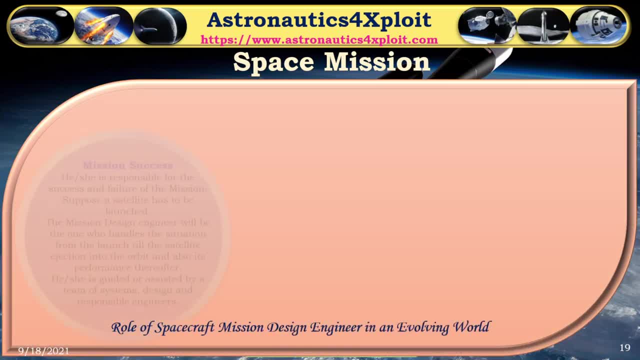 in the development role of spacecraft mission design engineer in an evolving world mission sources. mission design engineer is responsible for the success and failure of a mission. for example, if a satellite is to be launched, the initial design engineer will be the one who handles the situation from the launch till the satellite ejection into the orbit and also 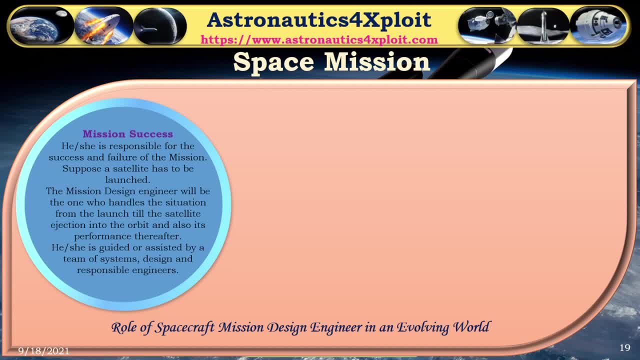 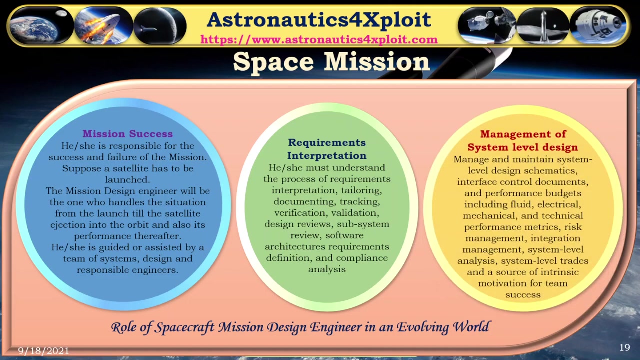 its performance. thereafter, ELC is guided or assisted by a team of systems design and responsible engineers. requirements interpretation: ELC must understand the process of requirements interpretation, tailoring, documenting, tracking, verification, validation, design, reviews, subsystem review, software architectures, requirements definition and compliance analysis, management of system level design. 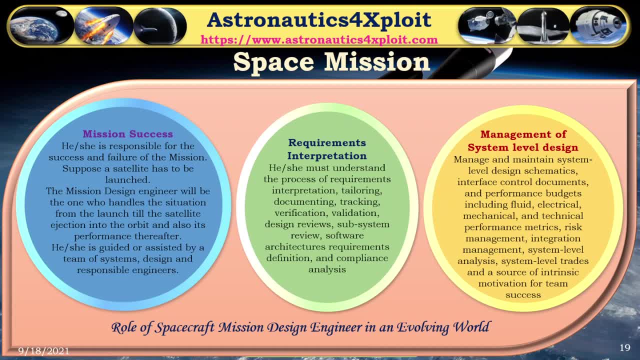 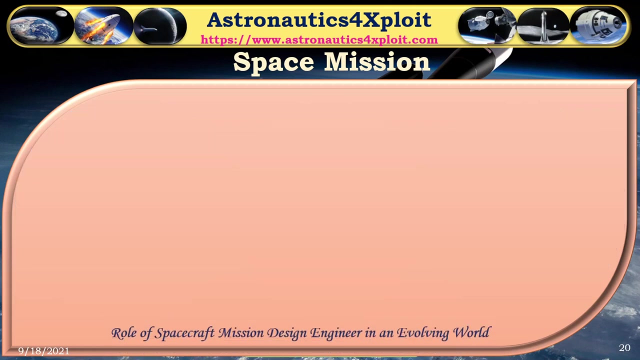 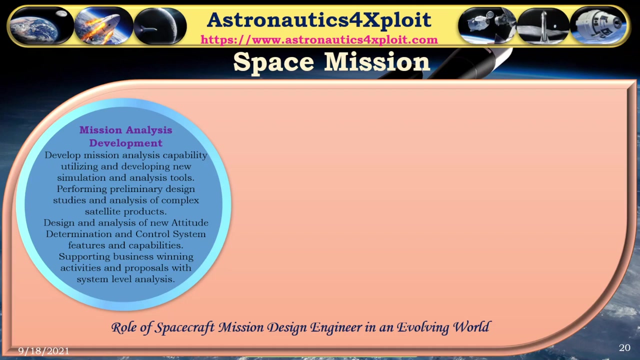 mission design engineer manages and maintains system level design schematics, interface control documents and performance budgets, including fluid, electrical, mechanical and technical performance metrics. risk management, integration management, system level analysis, system level traits and the source of interesting motivation for team sources. mission analysis development: ELC develops mission analysis capability, utilizing and developing. 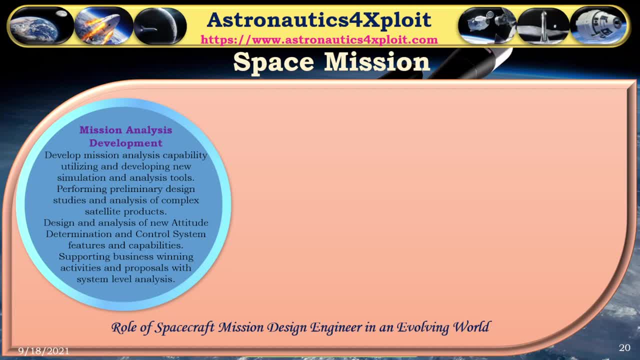 new simulation and analysis tools, performing preliminary design studies and analysis of complex satellite products. design and analysis of new altitude determination and control system features and capabilities supporting business winning activities and proposals with system level analysis. program reviews. ELC supports progress reviews and gates towards completion of projects on 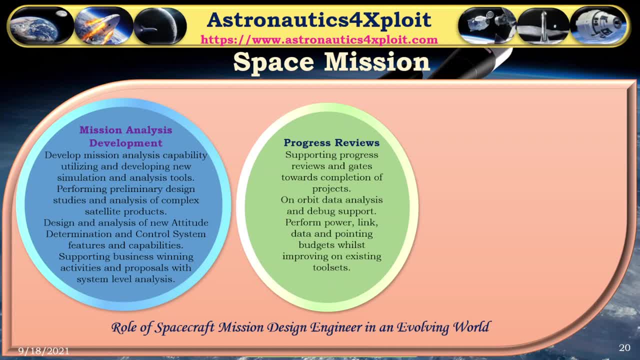 orbit data analysis and debug support. perform power, link data and pointing budgets, while improving on existing tool sets problem solving. ELC develops and applies advanced techniques for solving a variety of vehicle flight mechanics and astrodynamics of the mobility mechanisms, problems performing trajectory simulation and performance optimization. 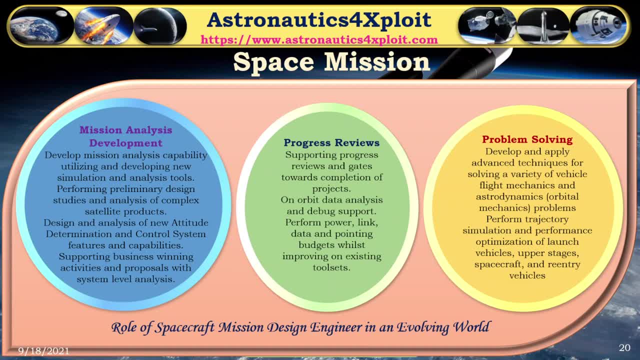 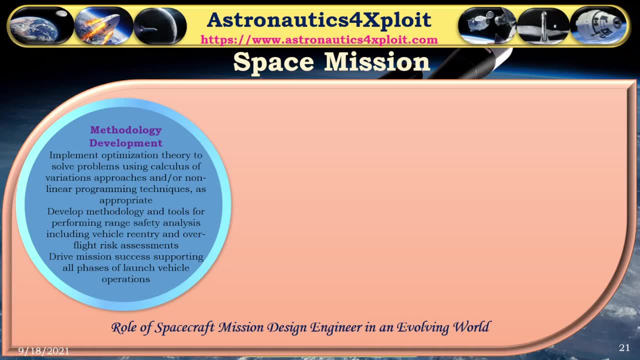 of launch vehicles, upper stages, spacecraft and reentry vehicles. Methodology development. He or she implements optimization theory to solve problems using calculus of variations approaches and run nonlinear programming techniques as appropriate. He develops methodology and tools for performing range safety analysis, including vehicle reentry and overfly risk assessments. drive mission. 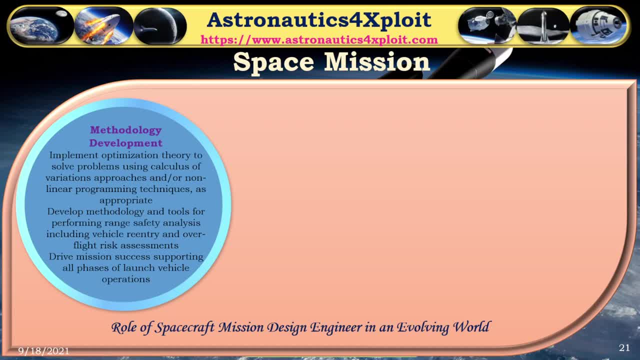 success, supporting all phases of launch vehicle operations. Parametric studies: He or she implements scripting techniques in order to perform parametric studies and continuation methodologies. utilizes numerical methods to analyze flight maintenance problems, including numerical integration, route solving problems and coordinate transformations. Results communications. 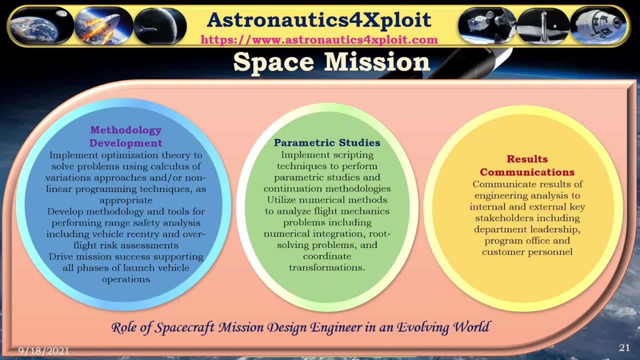 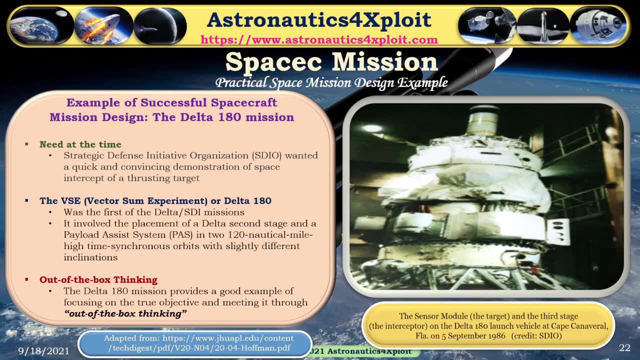 He or she communicates results of engineering analysis to internal and external key stakeholders, including department leadership, program office and customer personnel. Here is an example of space mission, Example of successful space craft mission design: the Delta-180 mission. The need at the time. 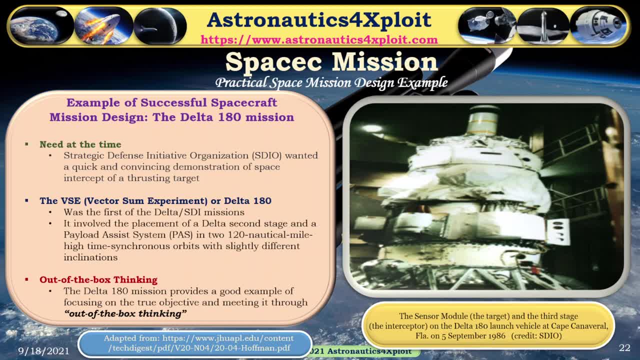 Strategic Defense Initiative organization wanted a quick and convincing demonstration of space intercept of a trusting target. The VSE was the first of the Delta missions and it involved placement of the Delta second stage and the payload assist system in 2, 1.12 nautical mile time. 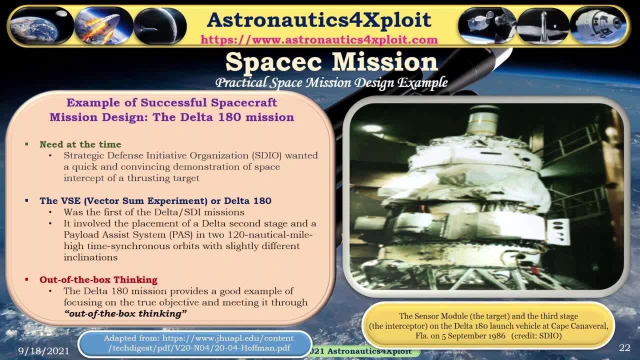 crop. synchronous operations orbit with slightly different inclinations, Out-of-the-box thinking. The Delta 180 mission provides a good example of focusing on the true objective and meeting it through out-of-the-box thinking. This picture shows the sensor module. that is the target and the third stage, the interceptor. 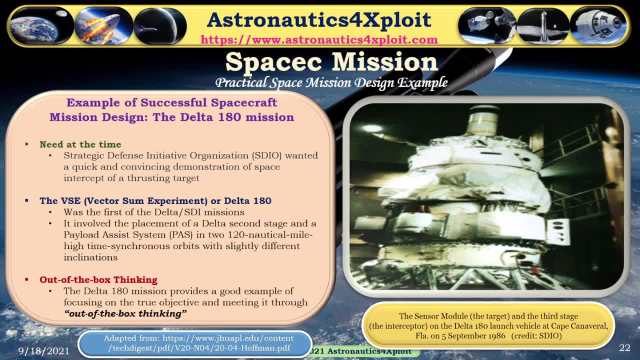 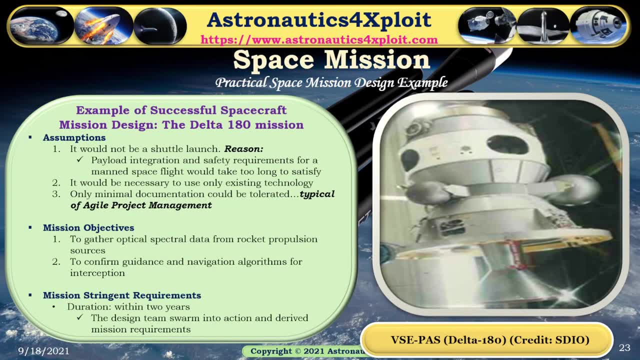 on the Delta 180 loaned vehicle at Cape Canaveral, Florida, on 5 September 1986.. Assumptions: The assumptions made were as follows. The assumptions are as follows: It will not be a shuttle launch, The reason being that the payload, integration and safety requirements for a manned space 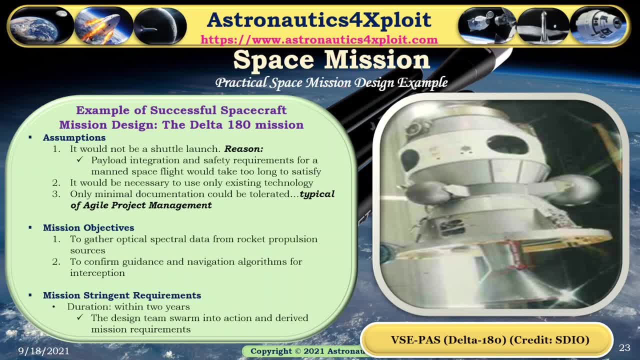 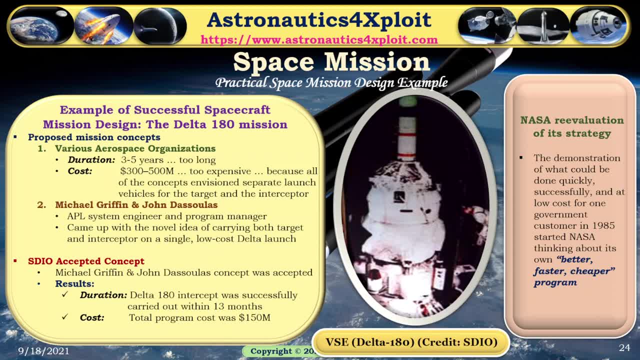 The other assumption is that the payload integration and safety requirements for a manned space flight would take too long to satisfy, and the cost was about 150 million dollars. all these are achieved through the combined effort of michael griffin and john dozalos, who came together as system engineer and program manager. 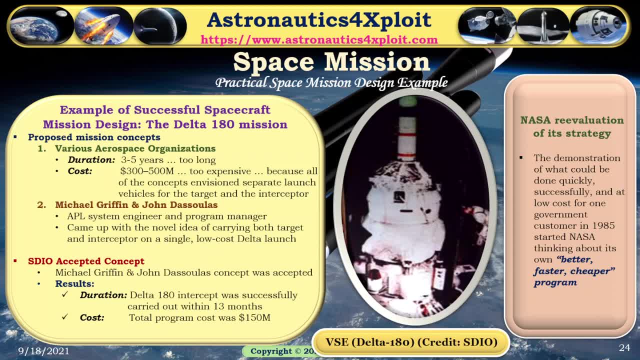 to see that new idea came in and they were able to save cost in the process. national re-evaluation of the strategy, the demonstration of what could be done quickly, successively and at low cost for one government customer in 1985 started nasa thinking about his own better, faster and cheaper program.